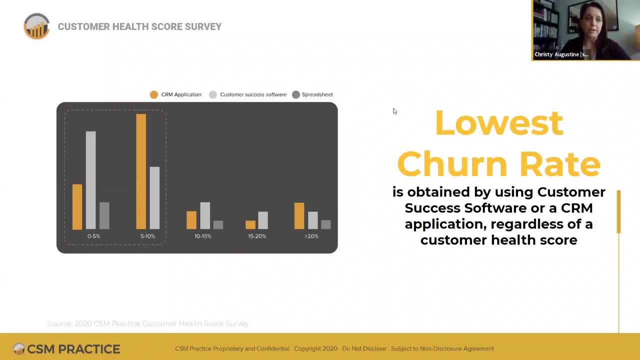 I mean I really want to know of the people who have 5% or less, you know churn, and we're in the spreadsheet bucket. Like what are they doing? Like I would like, would love to double click on that bar. I mean they've got, like, the desired results and they're in a spreadsheet. 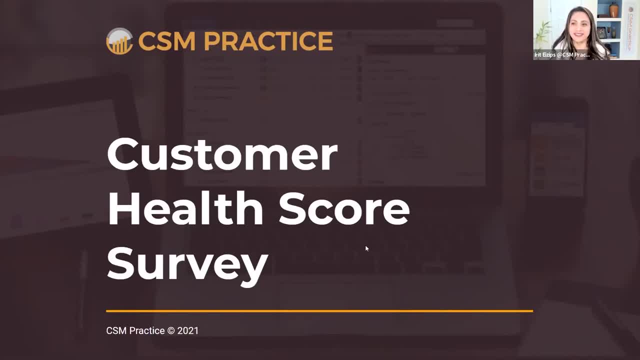 There's a lot of assumptions around customer success, health scores. Okay, Some of you might already think that they know the answer, So we did this survey. I'm really glad we did it, because even I learned something. So we had a lot of outcomes and statistical analysis. but I'm just 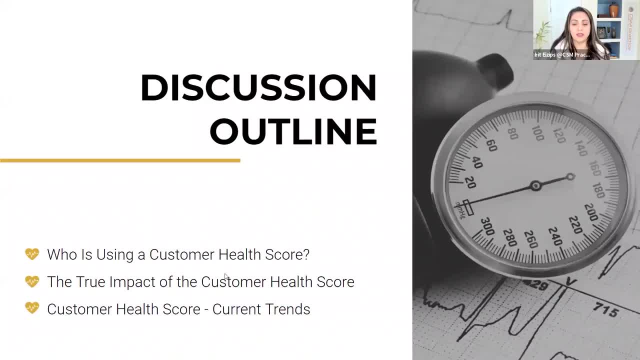 going to highlight the most interesting ones in my opinion. So we had three main themes that came out of that research. One is: who is using health scores And then what is the true impact of customer health scores? I think there's a lot of assumptions of what health score is going to benefit the 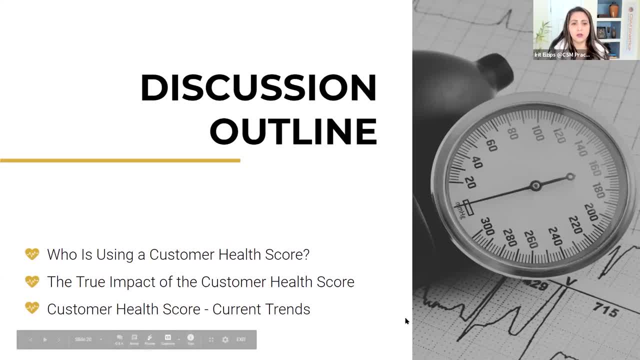 business. And then there's the reality. And then what are the current trends? You know what are people using, What metrics. you know how they're using it or how they are. you know updating it often. Before we start, I'd like to remind everyone: subscribe to our YouTube channel for 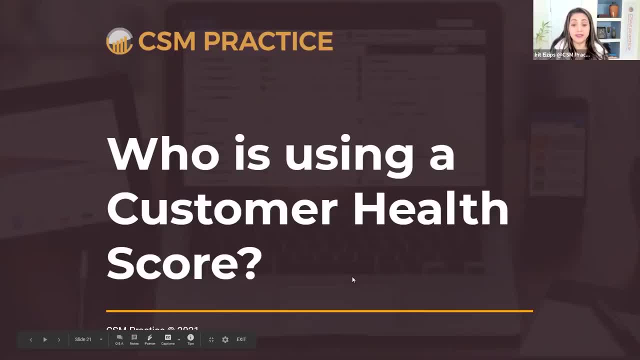 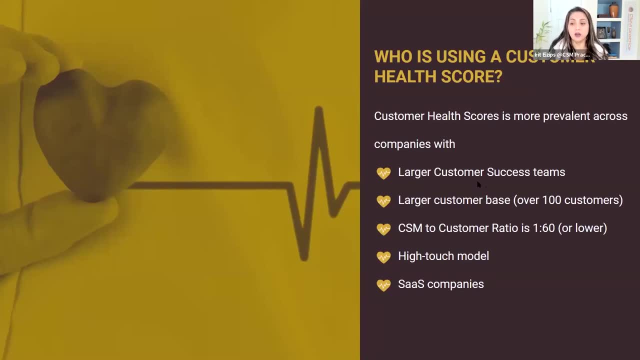 all the great videos that we produce on customer success, Who is using customer health scores? Some of it is not surprising. Okay, But it is more prevalent, Sounds like, in larger customer success teams. not surprising When there's a larger customer base. you know, over a hundred customers, obviously, But then 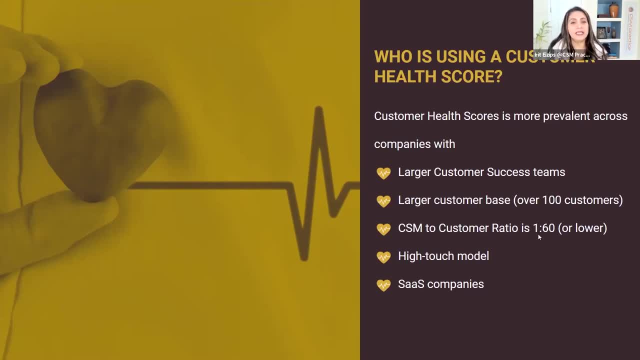 we found that when the CSM to customer ratio is below one to 60, so when it's one to 20,, one to 10, one to 30, there's more aptitude for customer health score, You would think. the other. 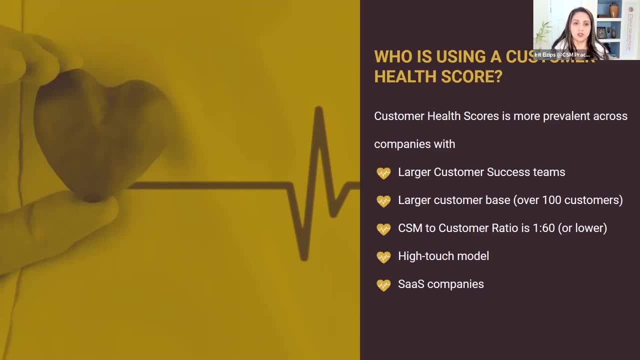 way around is like: oh, the more customers each CSM manages, the more it makes sense to have a customer health score, the more it is maintained. It's actually the other way around. So the lower the customer ratio, the higher touch model. 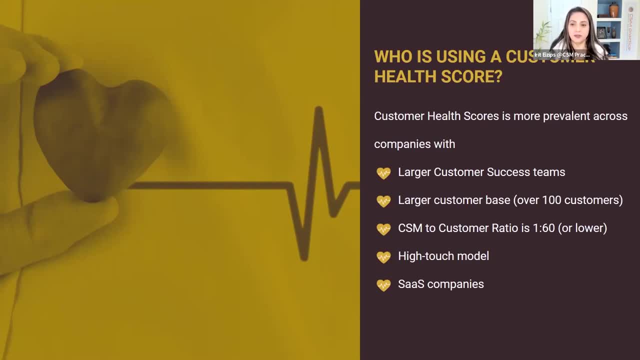 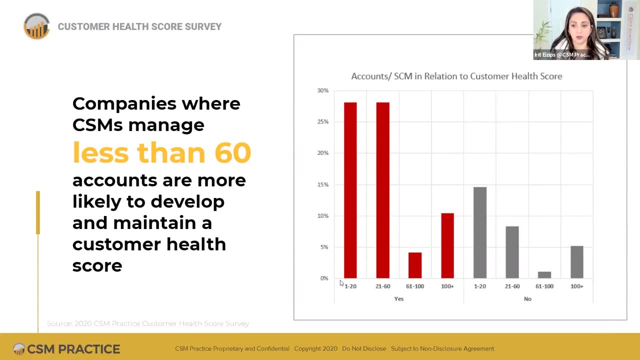 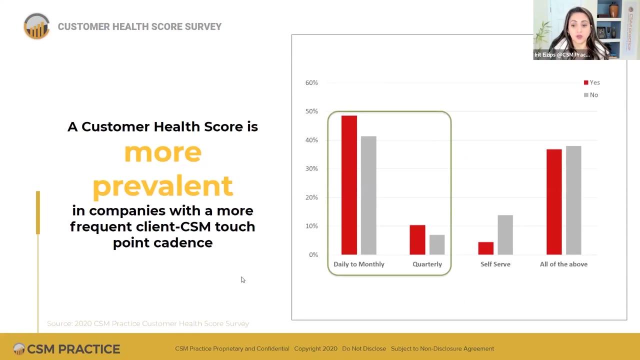 the more prevalent customer health score seems to be. So actually, so this is the ones that said yes had like predominantly a lot lower customer engagement. So 60 and below 60 is like the prevalent when we had the health scores, And then it's also more prevalent when the touch point is. 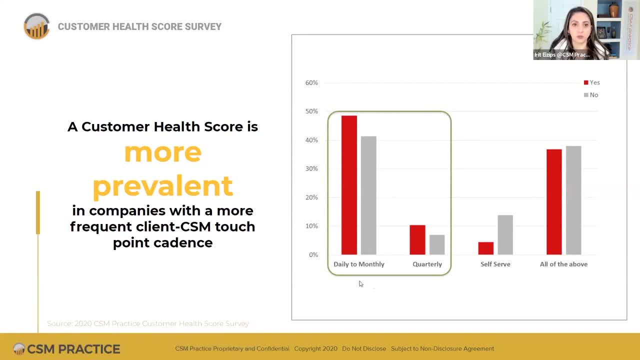 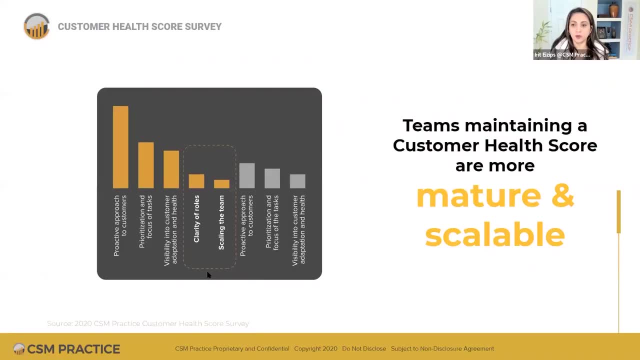 more frequent. Some of the organization had all engagement models implemented, So it was hard to see. the high touch models had customer health scores And then the true impact of customer health scores. teams maintaining customer health score are more mature and scalable. So here's what we asked them: What are your strengths as a team? 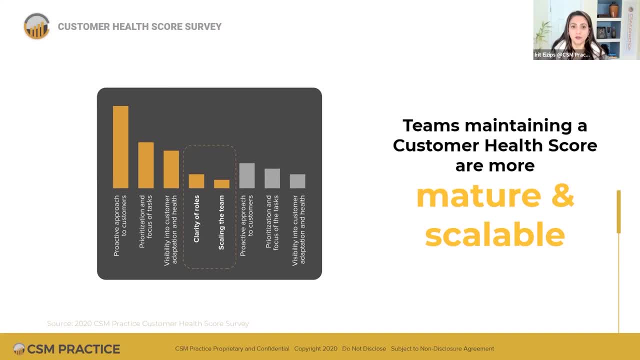 And we were expecting that customer success teams that had a health score have better attributes, like they're more proactive, they're better at prioritizing tasks, that they have better visibility to the customer adoption Overall health, but we had the exact same strengths from those who did not have a health. 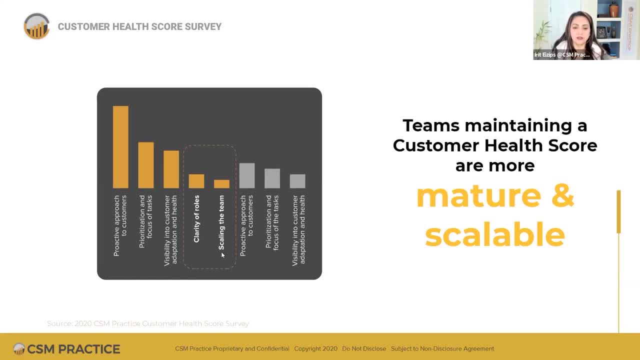 score. So the only thing that we found as a differentiator is that these two popped up as major strengths, which is clarity of roles and the ability to scale the team, And I think that this has to do with a lot of times, like the majority of the teams, that had a health score. 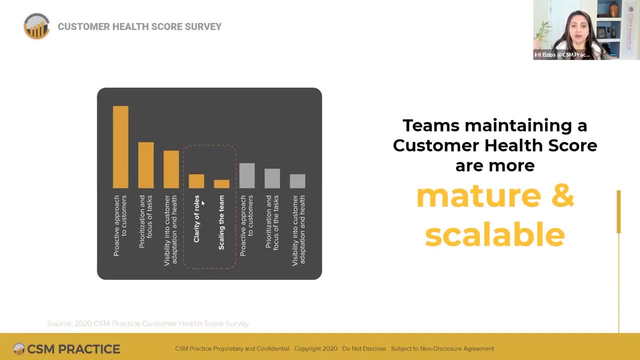 actually had a CS technology and clarity of role. If I have a health score, I know what my metrics are And so I'm more clear around what it is that success means. If you think that you're going to do a health score and be more proactive and have the team better prioritize the no, they're both very 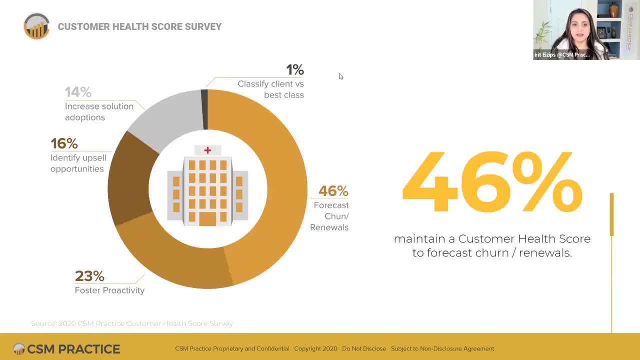 strong at that, So that's really interesting. So we asked about: why do you maintain the customer health score? 46% of them did that to forecast churn and or renewals, 23% to foster productivity. Now we already know that that's a moot point. Identify upsell opportunity: only 16% Increased. 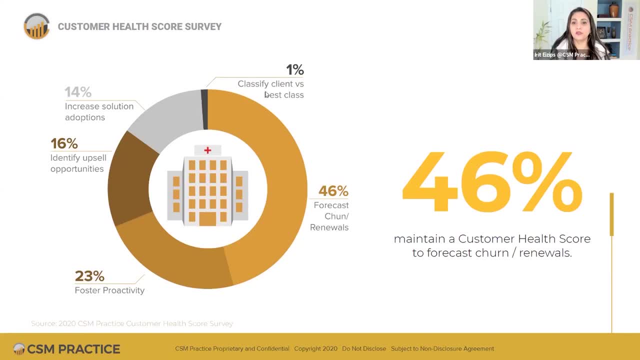 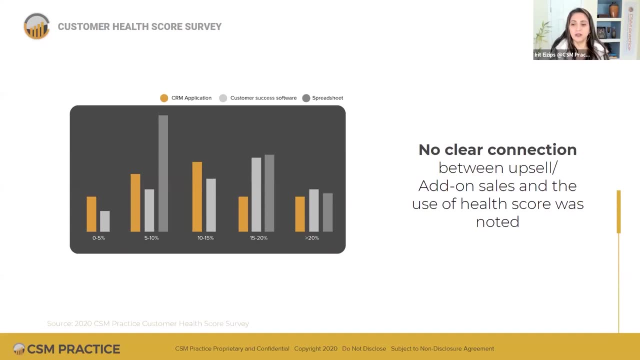 solution adoption: 14% And 1% to classify client versus best in class. The sad news is that we didn't find a clear connection between the ability to upsell or do add-ons to the use of a health score. No connection, So if you have a health score, it doesn't mean that you're going to have. 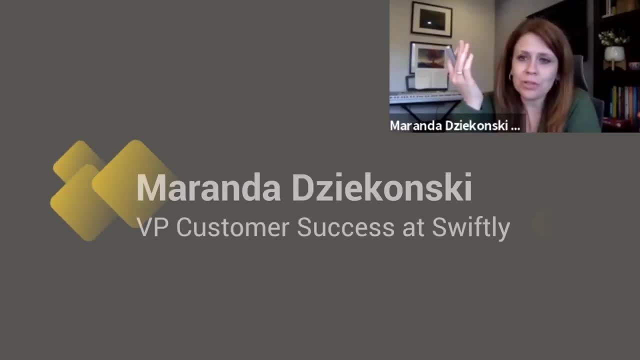 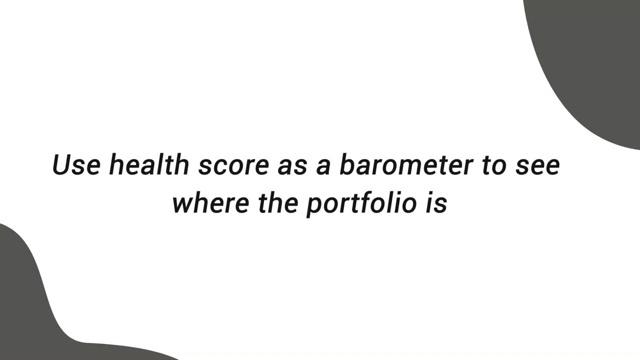 better upsell and cross-sell opportunities. I think health scores are just not as scientific as we think. There's just so much art to it. I use it only as a barometer, just to kind of see where the portfolio is based on a few key things. But 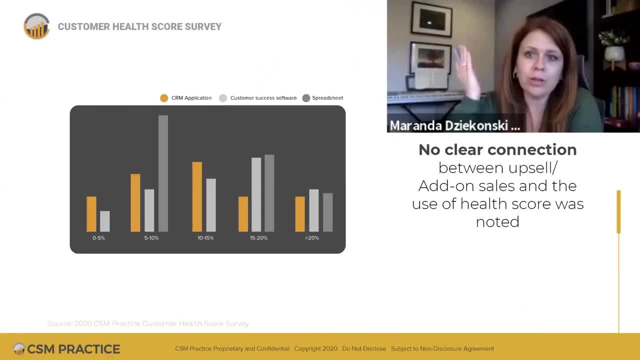 let's be real. We've all had customers who are very healthy, churn or who have the health score model that we spent so much time building out renew, and they were at the other end of that spectrum. So I just find this so fascinating. 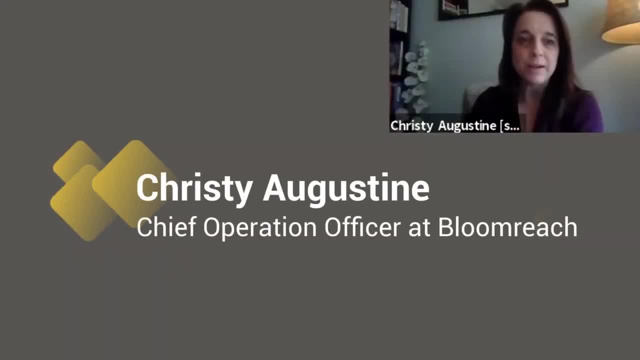 Totally, I agree with you. I'll tell you, we recently kind of started to deprecate it, because 50% of our accounts were red but north of 95% of our accounts were renewing, And so you just couldn't correlate, And so we've started to switch over to some other metrics to 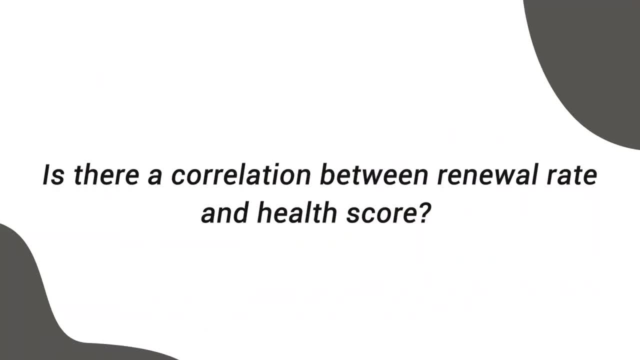 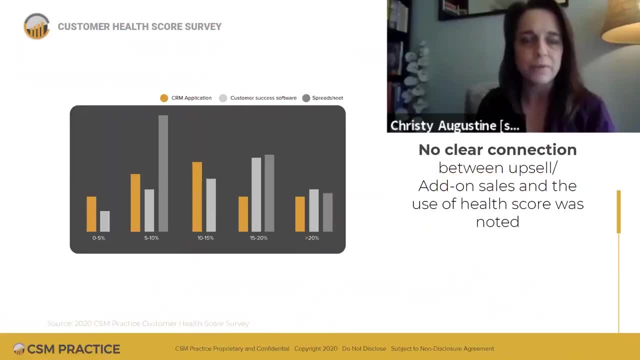 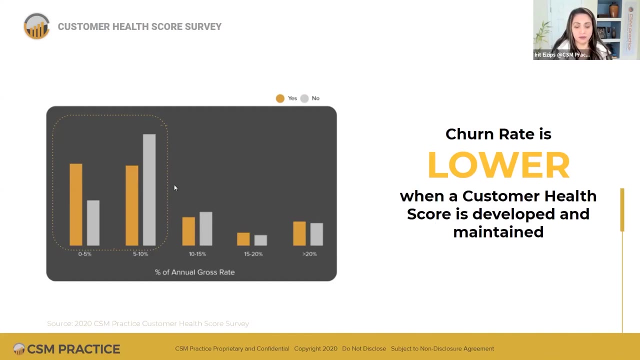 kind of correlate particular risk factors or upsell, And so I was wondering if there was that data on correlation between a renewal rate at a company and a health score. Churn rate was lower when a customer health score was developed and maintained, And not only that. so this is the group you can see with the yeses they had overall, but everybody. sort of like had. it wasn't very consistent, but we did find that if they were impacted, whether they had a churn issue or not- if you did have a customer health score, you would have a lower increase in churn rate in 2020.. 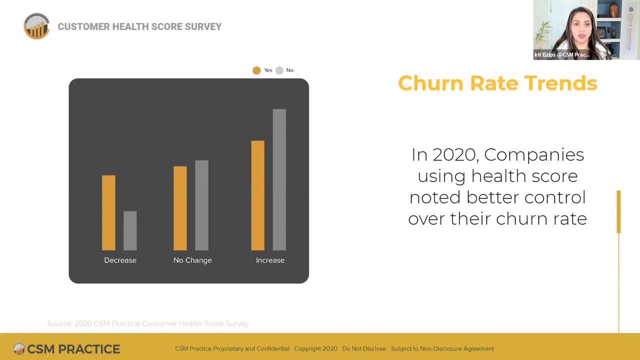 Because we knew that churn rate went up for a number of reasons, regardless of health score or not. but were you able to have better control over it If you had a health score? if you decreased, you decreased it more. If it increased, it increased less. So I thought that was really. 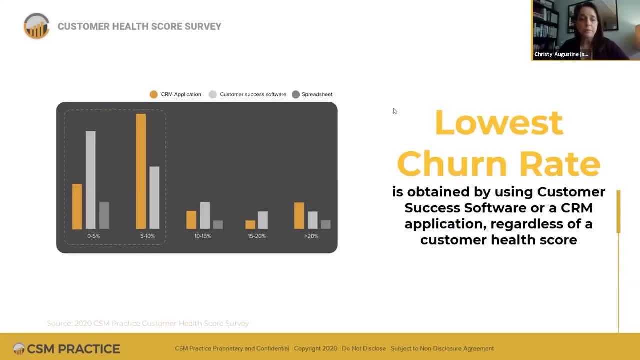 interesting to see. I mean I really want to know of the people who have 5% or less churn and were in the spreadsheet bucket. like what are they doing? Like I would love to double click on that bar. I mean they've got like the desired results and they're in a spreadsheet. It's like who is that? 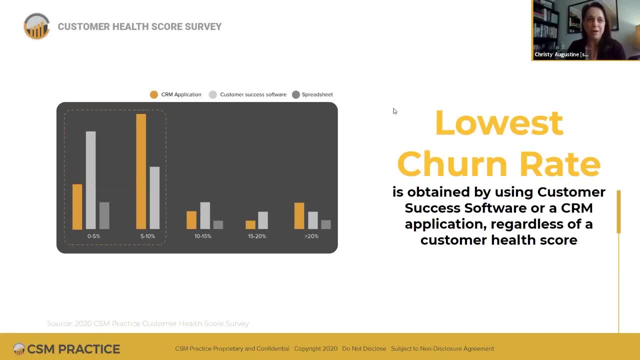 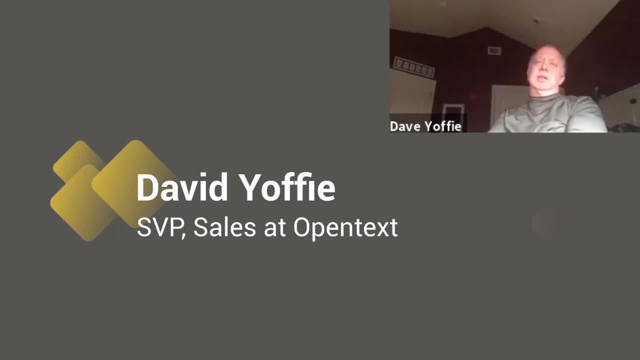 And like what I want to know. like, are they doing something even better? What are they? what are they up to? They stole a million dollar product and the company stuck with it. Yeah, They're lying. How much commonality do you think there is across this about what a health score is? 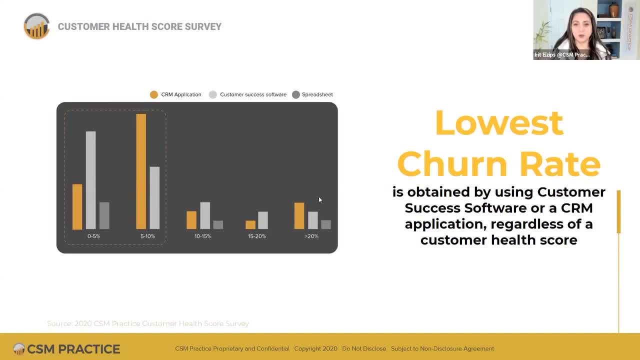 So we did ask: what did they include in the customer health score? We just didn't know. I mean the best we could do in a survey, obviously, but my guess is that a lot of the times the health scores are not optimized or not done in an optimized manner, which is one. 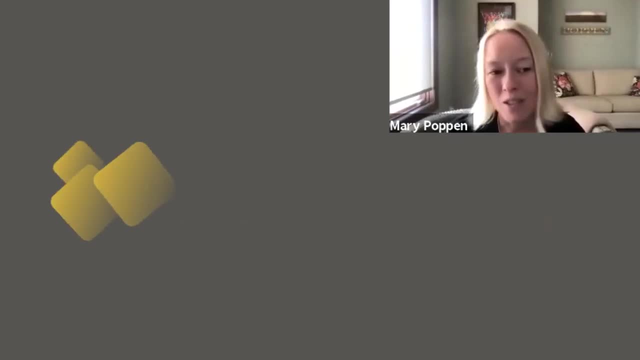 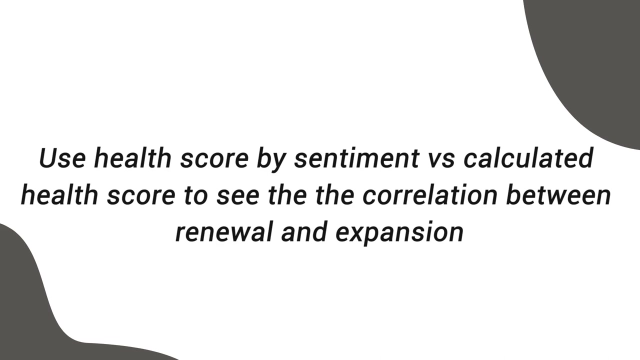 of the conclusions that I think that I have from this survey. So it'd be interesting to look at too, like sentiment, So the health score by sentiment versus the actual calculated health score, and to see, you know, the correlation between renewal and expansion of how well the CSM, because in a portfolio less than 60, let's just say 10. Ideally, 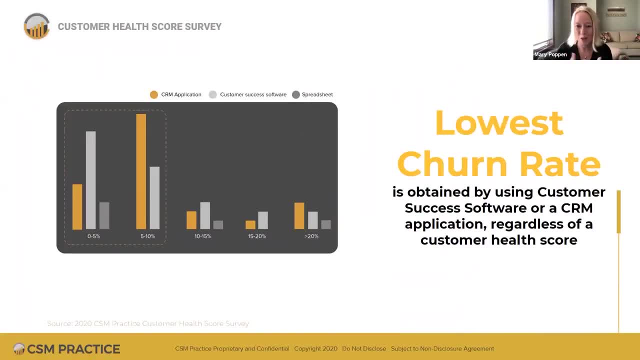 they're close enough to their customer that their health sentiment should align to those other key metrics, Whereas when you do have a portfolio of a hundred or more, you know the CSM sentiment probably doesn't mean a whole lot in comparison to adoption and some of the other calculated you know pieces. 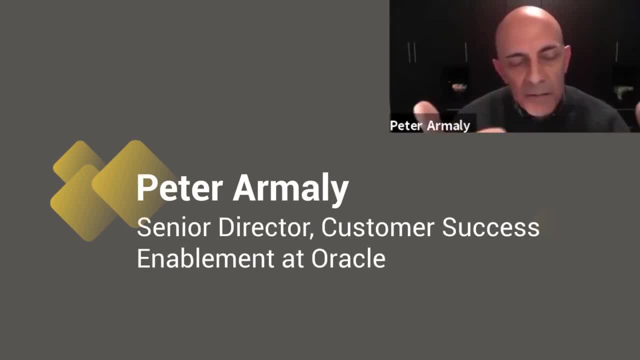 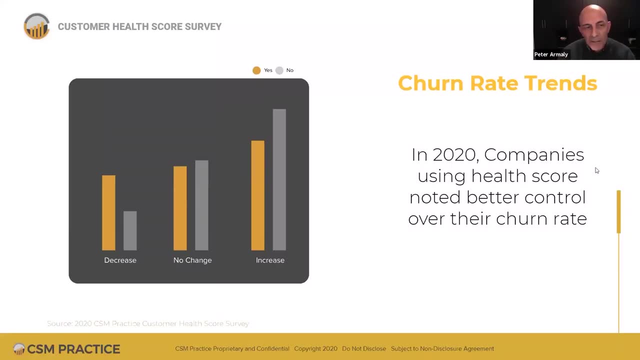 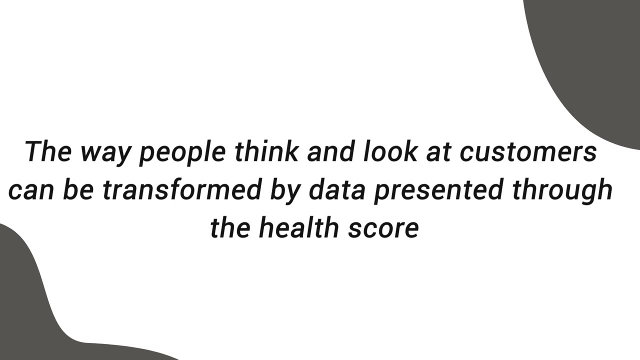 Health scores are valuable because I see them as an instrument to drive conversation inside a company. So customer success should lead the way and say: we've arrived at this measure of assessing our customers. Do you agree? And most of the time, most of the time, people don't don't agree with that. So you have a conversation and I think 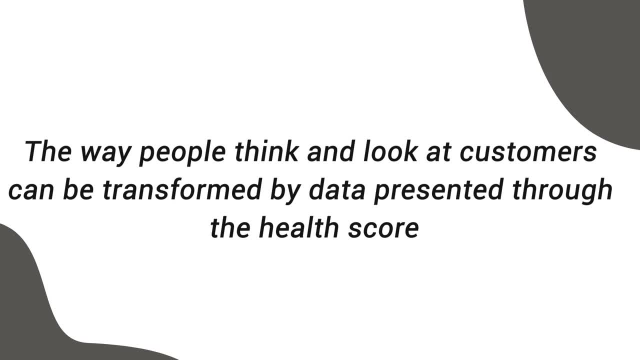 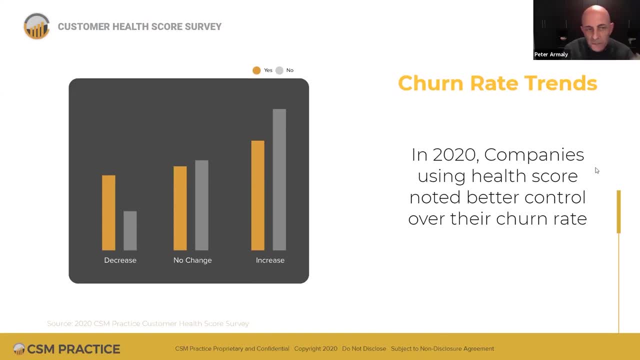 it can help transform the way people think and look at customers through data that's presented through the health score, And so that's kind of the way I'm thinking about it And when I'm helping to influence a little bit, that Oracle's developing a little more sophisticated one. Now we're 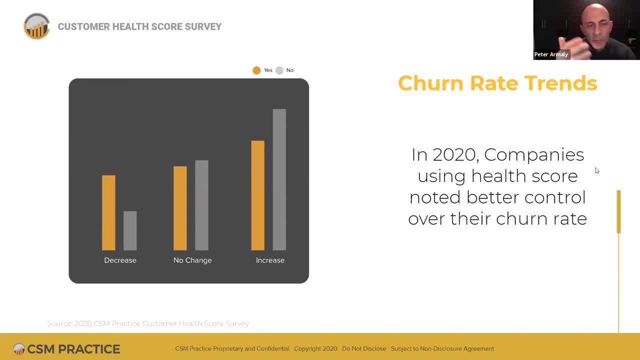 encountering that right now. So sales doesn't agree, you know, support more or less agrees. Marketing is kind of out of the picture. So you know what I mean. Like there's a conversation that can be had using the health score, I think, as a, as a, as a device to transform the objective of 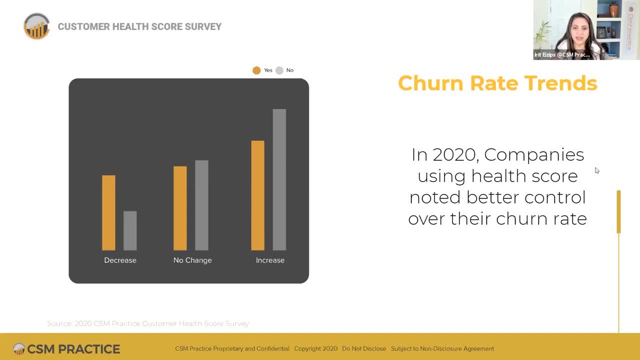 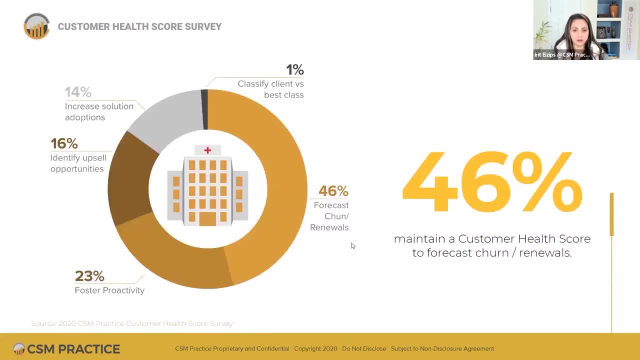 why we're doing customer health scores And I think the main issue right now that we have- and this is why it doesn't- there's no correlation, There's four correlation. It's because you know this question. why are you creating it in the first place? 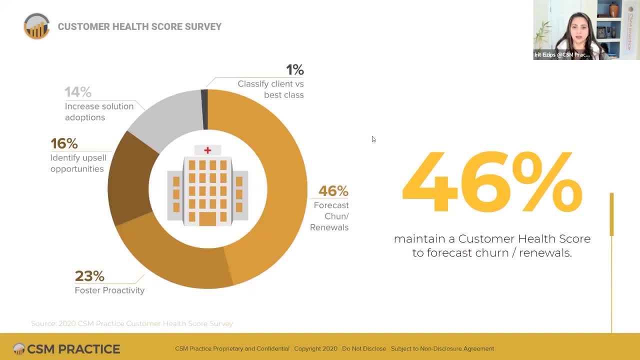 I think it's all the wrong reasons. If we could build a customer health score to develop these internal conversations or even external conversations with clients, then the health score looks different And it's not to say: are they going to churn or not. It's really about: are they becoming best in class Or 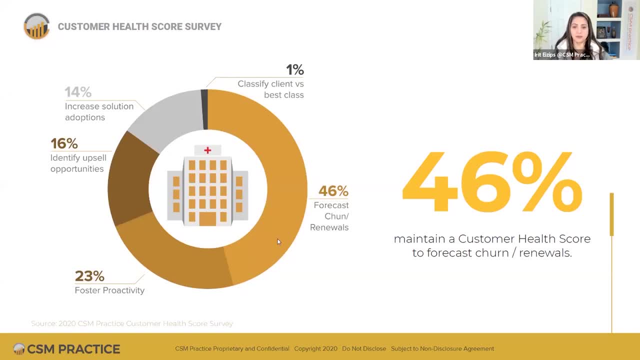 what else should we be doing strategically to help our customer base become successful? But you can see how many of them are using that. I know it shows you, So I think that's really what the the Hummel way for me is like. okay, 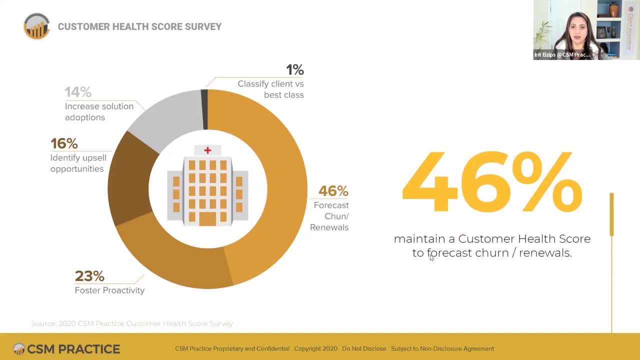 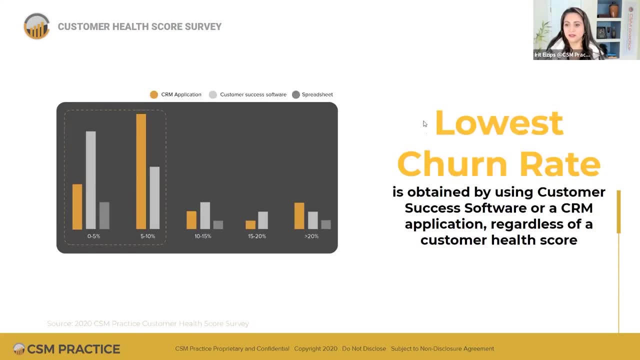 they're trying to forecast better, but you can't do that. There's just so many things that influence a, A renewal, a decision. Let me show you a few more things. The lowest churn rate, you know. like we cause, we asked what, what's your churn rate? And so we wanted to see if there's a. 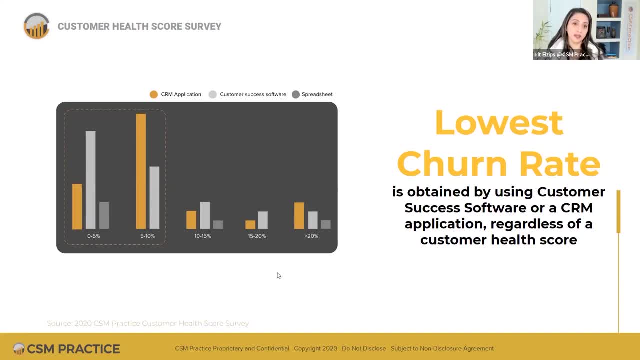 correlation If you had a low churn rate because you had a health score or not, not so much. we couldn't find correlation there. So then we said: well, what if you know, for those who did have a churn rate, which ones have the lowest one? And the only correlation we found is that if they 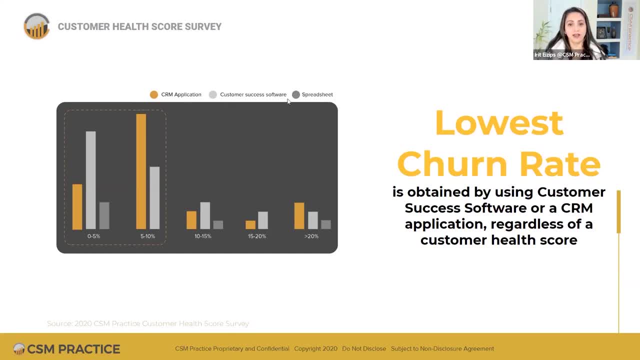 were using, Yeah, A CRM system or a customer success software, they received a lower churn rate, regardless of whether or not they had a health score. Can you just imagine- And again I want to make sure that I got that, It's like you're- you're saying they had either. 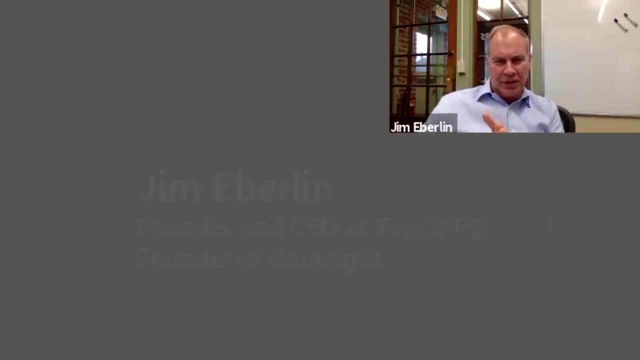 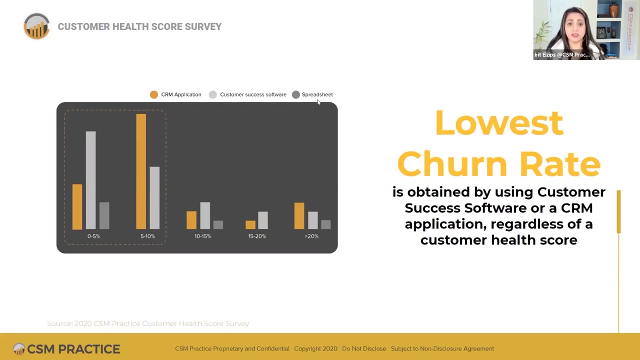 a CRM or customer success as opposed to a spreadsheet. Is that what? Yeah, Some teams don't have, they don't use the CRM application, They don't use a customer success software and they have everything in spreadsheets. If they're using a customer success solution, or or. 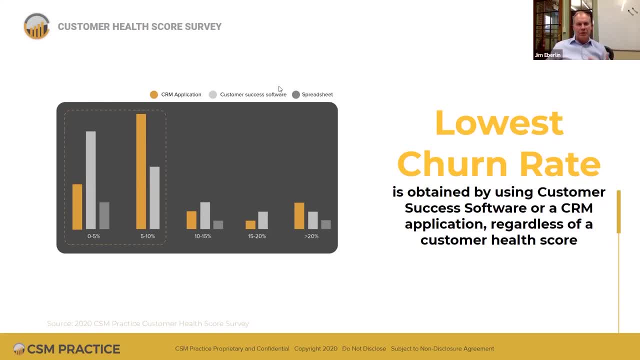 Or even a CRM solution. they're just going to be more apt to good, healthy processes doing this kind of stuff versus just doing it. Yeah, So if you look at the lowest bracket, you're at the 5% churn rate. 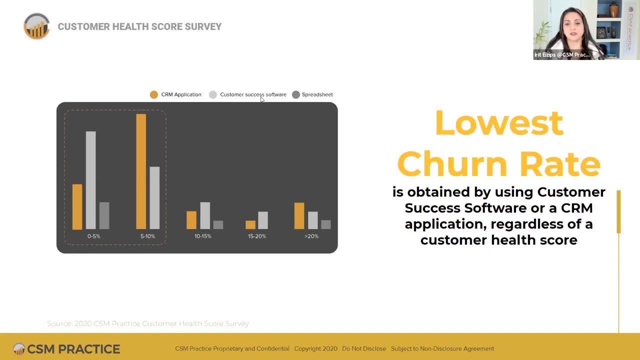 the dominant ones are the ones that have a customer success software. Oh yeah, Honestly, I think it's all about visibility across the organization. you know, so product knows where to go to get information and sales and CS, and you know it's just making sure everybody's. 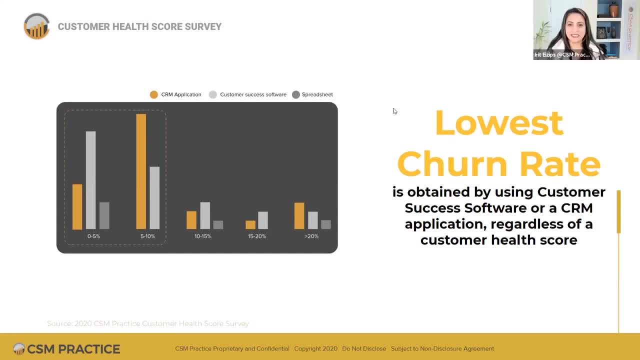 talking the same language and doing the right things, But isn't it surprising, like a little bit? like, Yeah, it is. It's kind of reassuring to see, though. Yeah, The reason we did that is that we want to have executives make decisions better. 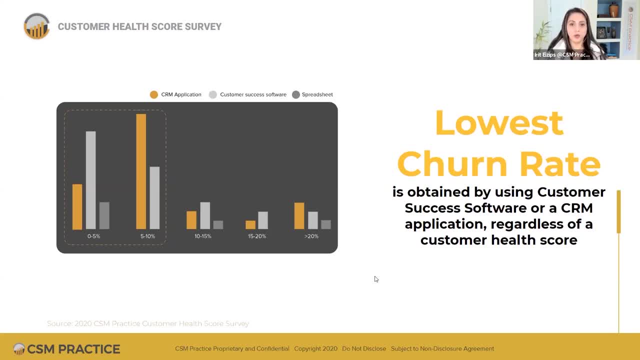 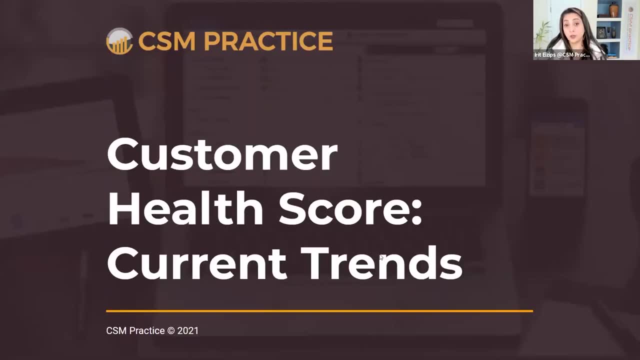 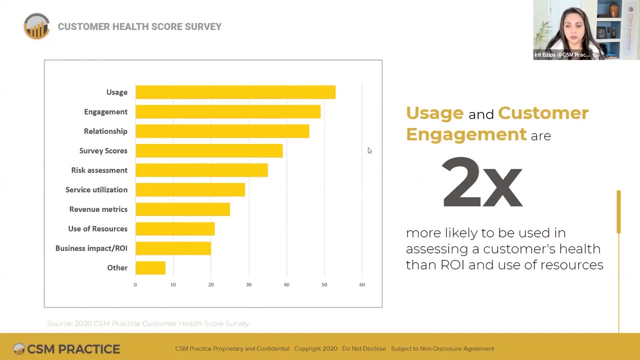 And if you could see across 200 companies what is predominantly recurring themes, then you can come up with some conclusions and avoid some mistakes. All right, So current trends: how do people use customer success health scores, if they have it? So we asked them: what do you include? What metrics, what components do 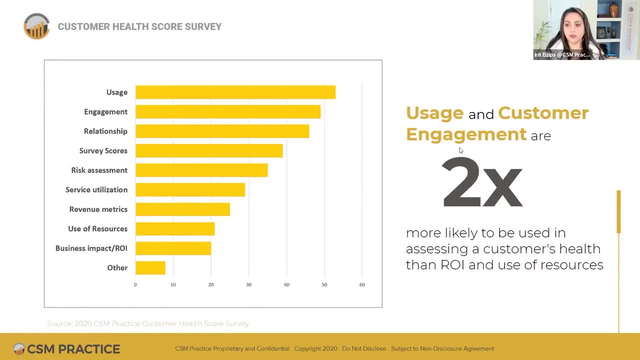 you include in a customer health score And we found the usage and engagement are twice more likely to be used uh versus anything else to assess the customer health score And, as you can see, like it's quite as much as ROI, which is interesting, I think. I thought that we you know. 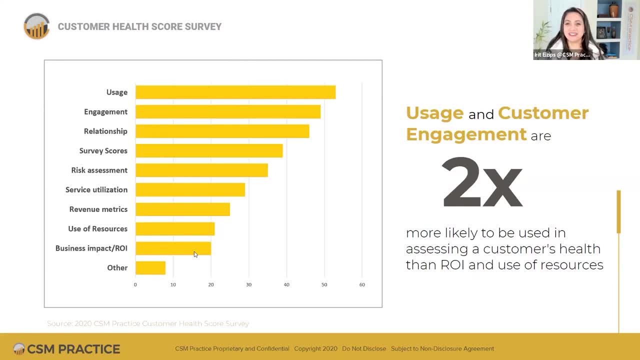 business impact would be one of the first things. you know how much value they're getting. No, it's like usage, but not as much. Well, here's the thing. I think that most of the customers would use their data and they would be able to write their goals on it, And sometimes, 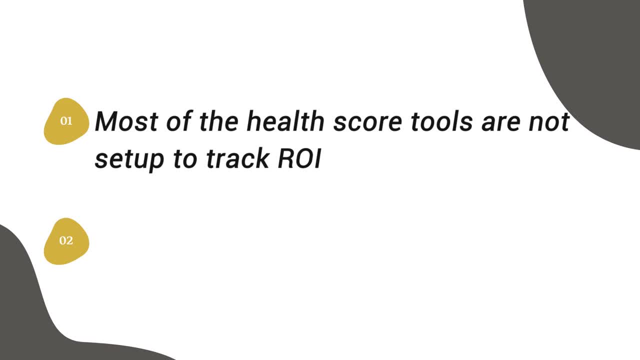 customer health score. tools aren't set up to track ROI. I think that's part of the problem. A lot of the tools are really heavily focused and make it easy to use certain formulas which are heavily focused around usage engagement, your manual relationship setting. 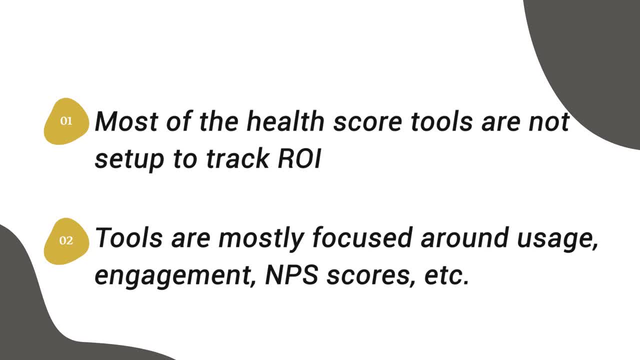 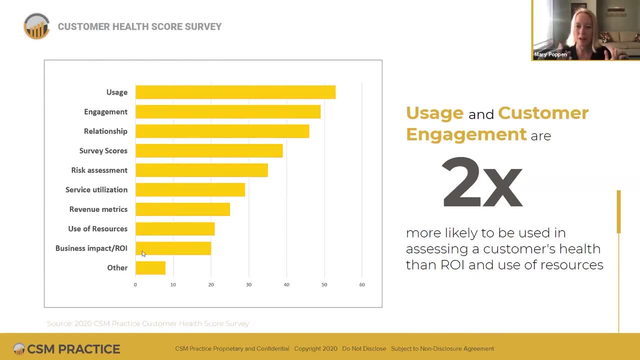 NPS scores. all of that. That makes sense to me based on what I know about the tools in the market. A lot of times I feel like we come up, we aggregate something or come up with something in order to educate the rest of the company to NPS the health score They're just glommed on to. 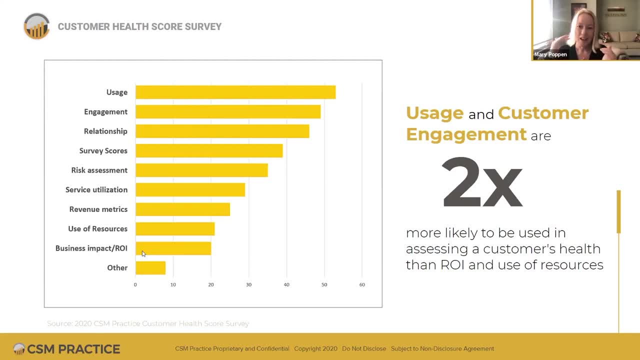 by other leaders. They can understand. health is whether the customer is red, yellow, green, All the stuff underneath it is really the most important. It just makes me think: are we doing a bit of a disservice to report on just a couple of key factors, or would we? 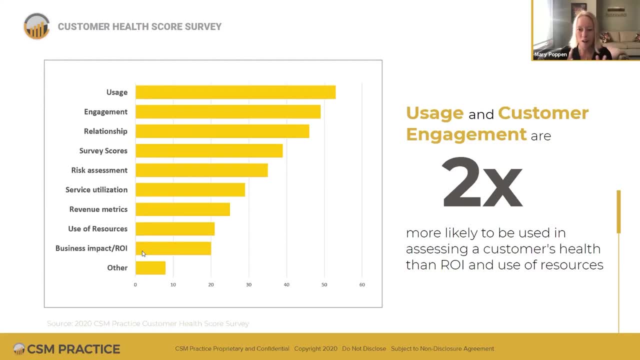 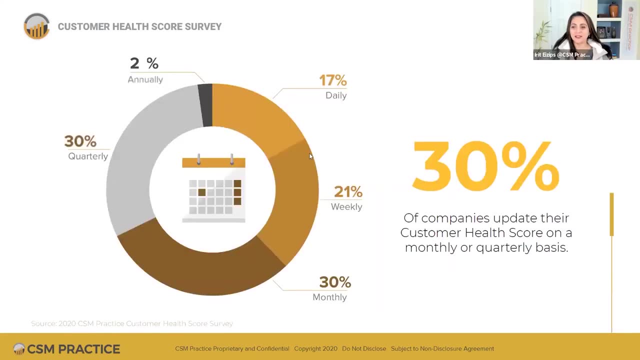 be better off Sharing a scorecard, maybe in a way that others can understand, but it's not pinning it to maybe just a score. Let me ask companies, your team, how often do you update the customer score? How often do you update it? That was interesting. Two percent actually do it annually. Most are. 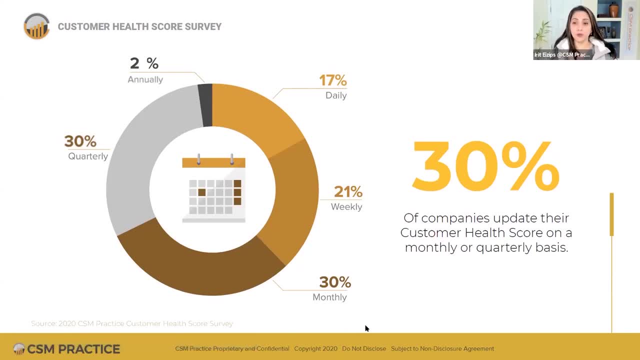 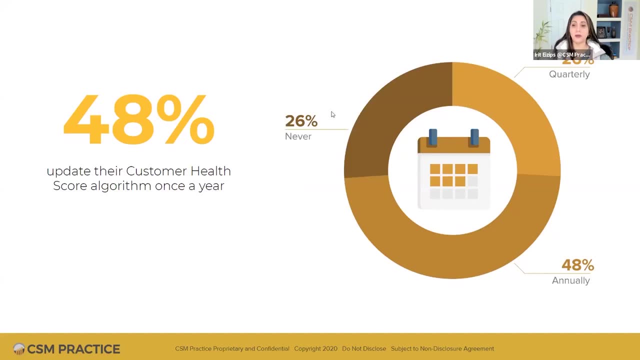 either doing it quarterly or monthly. Now remember that most of the people or most of the companies with health scores have a high touch model. Then we asked them about the algorithm: 48% update their algorithm once a year. 26% never set it up, forget it. Then 26% quarterly. I think that